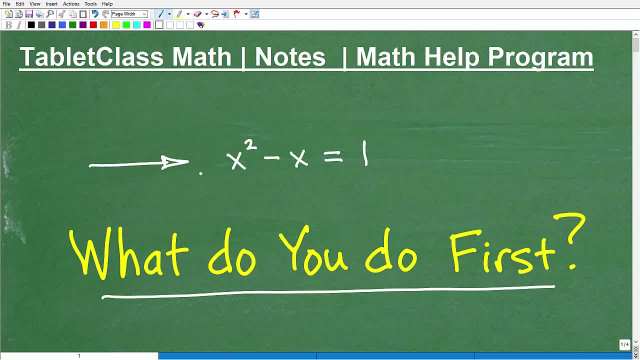 algebra part of your course. you're going to need to know this. Now, what are we talking about here? Well, we are talking about equations, And in algebra there's different type of equations. But this little thing right here, right, there is a clue, Okay. so I'll give you a little bit of a hint. It starts with the Q. Okay, what type of equation are we dealing with here? It starts with a Q- Drumroll, please. Okay, here is the answer. This is a quadratic equation. Okay, so we're talking about 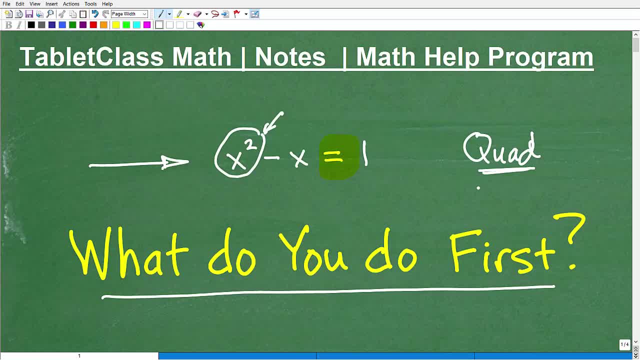 quadratic equations, And if you are still lost, then you're definitely going to want to watch the rest of this video. But we're going to be solving this particular quadratic equations, And when you solve quadratic equations, there are some specific first things you need to do, especially when the equation that we're looking at is in this kind of form. Okay, so we're going to talk about that Because, think about it, You know what steps you take. your initial steps is like what path you're going to be taking. 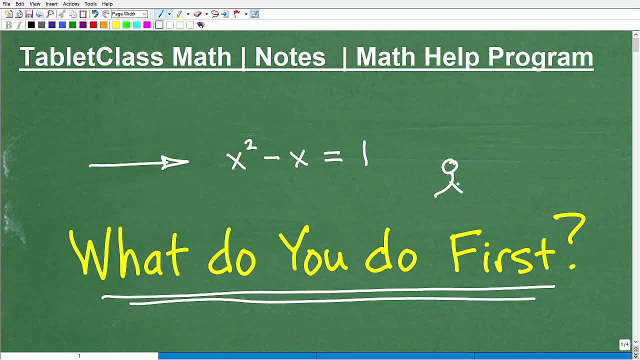 like what road you're going to go on. So if, here, you are right there and you're like: okay, what's the first thing I do? Well, if you do, if you get on the right road, okay, like, okay, you do the right first step and then you can take the right second step And you're right on, you're on a right third step. well, then you're going to go. eventually you're going to get to the solution. Now, if you take the wrong road, okay, guess what, you're going to take the wrong first step And then you're going to take the wrong second step And then you're going to end up in the land of confusion and wrong answers. So we don't want. 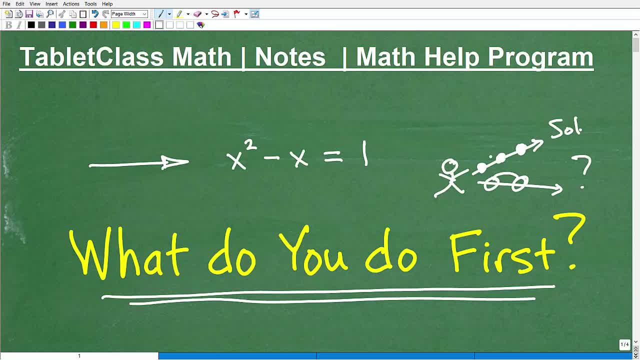 that to happen. So we're going to talk about things that you didn't want to be really aware about when you're dealing with quadratic equations, something like this, And we're going to get to this in just one second. But first let me quickly introduce myself. My name is John. I'm the 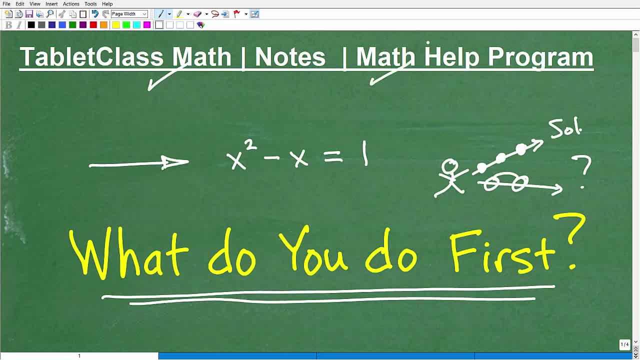 founder of tablet class math. I'm also a middle and high school math teacher And over several years I've constructed what I like to believe is one of the best online math help programs there is. Of course, I'll let you be the judge of that. If you're interested, you can check out my math. 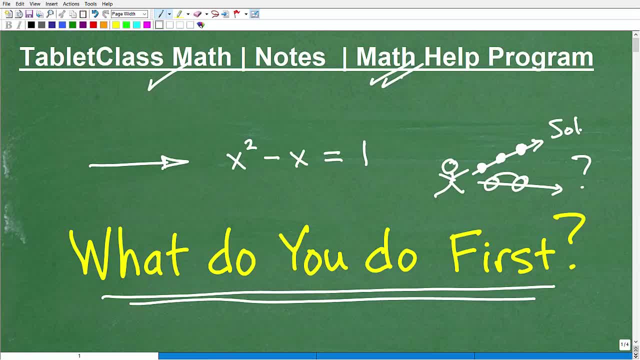 program by following the link in the description of this video. But basically I have 100 plus different math courses, ranging from pre algebra, algebra one, geometry, algebra two. I'm going to be launching pre calculus here shortly, But I also have a lot of courses in the area of test. 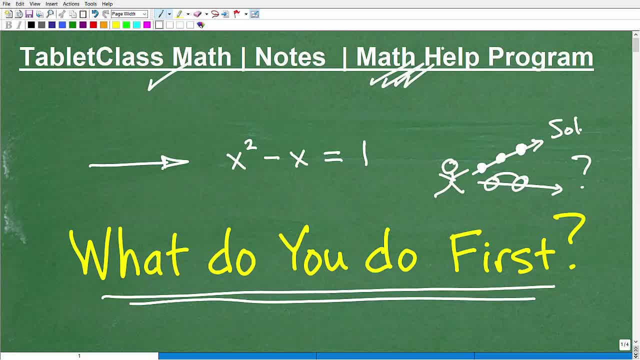 preparation. So if you're studying for the GED, HiSET, TASC, SAT, ACT, GRE, GMAT, ASVAB, ACCUPLACER, ALEKS exam, CLEP exam, maybe a teacher certification exam, all those exams. 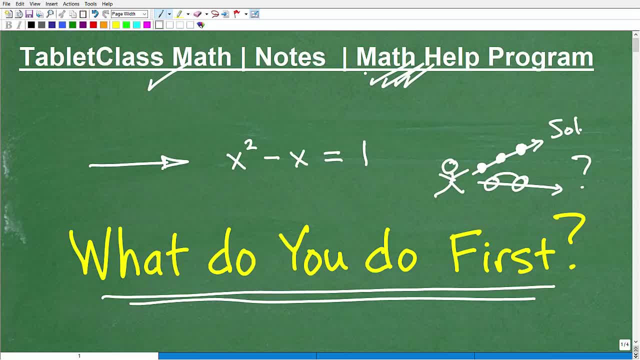 maybe a nursing entrance school exam. All those exams have math on them, And if you don't do well in a math section, you don't do well on the exam. So let me help you prepare. Just go to my website, check out my full course catalog. I should have your exam Now, if I do not drop me a line and 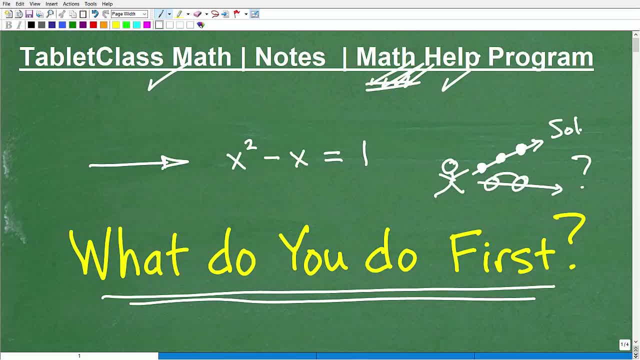 I'll help you out the best I can. I also do a lot with independent learners like homeschoolers. So if you homeschool, I have a great homeschool learning system And I obviously help those either just having a tough time in your current math coursework or you're just having a tough time. 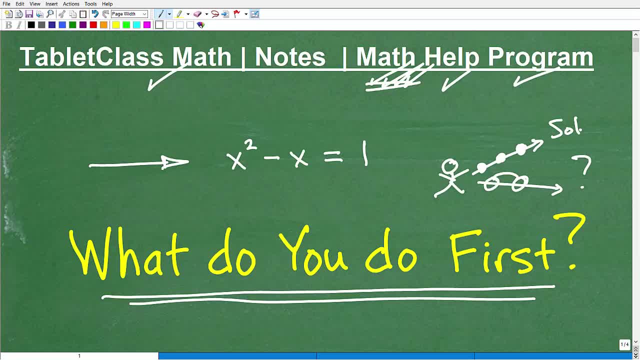 with your courses Now. if you are serious about wanting to do better in math, okay. if you're not serious, just disregard this part of the video. But if you truly are serious and motivated to want to get better at math and overcome your math struggles, then you got to be serious about this. 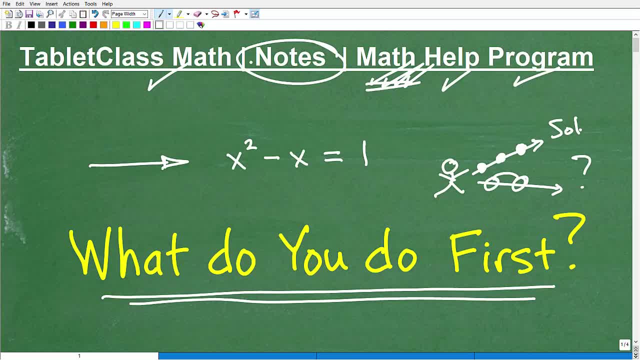 and that is note taking, Okay. so, over decades of teaching mathematics, one thing is apparent to me: those students who take great math notes almost always end up looking like this at the end of the school year. And the reverse is true: those students who take great math notes almost always end up: 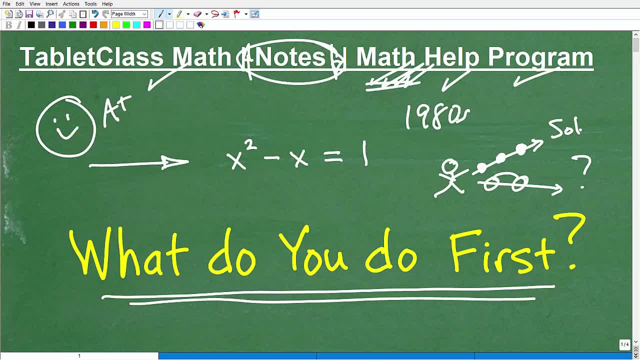 looking like this at the end of the school year. And the reverse is true. those students who take great math notes almost always end up looking like this at the end of the school year. And the we're like me way back in the 1980s. What was I do doing back there? Well, I was taking notes. 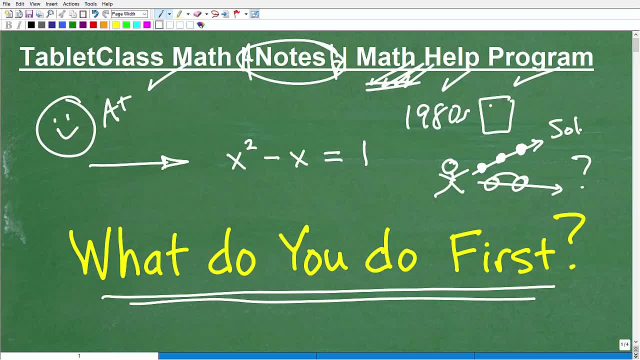 but they had nothing to do with math. I was like writing to my buddies: hey, what are we doing this weekend? We didn't have any cell phones or texting or all that stuff. We just literally, like you know, try to do whatever we could to not get caught by the teacher, Because back in those 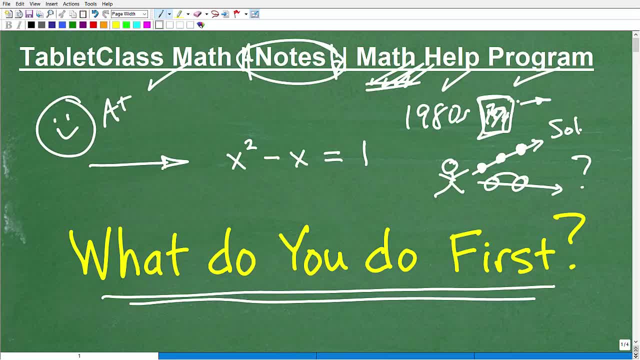 days they would, I mean, they would throw us in detention. I spent a lot of time in detention But at the end of the year, what kind of grades that I get. I would get like c minuses and i would look like this and we'd like, why did i get this grade? uh, well, you know, obviously i 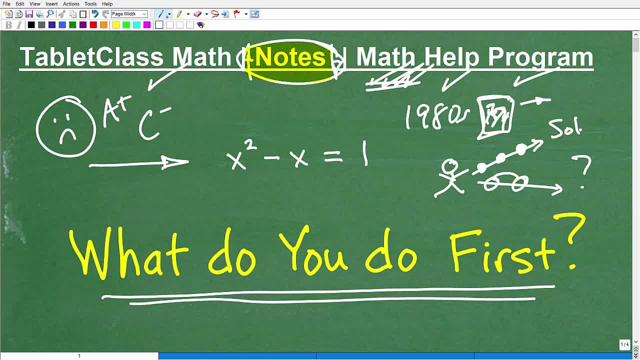 wasn't doing what i was supposed to be doing. so take a look at- take a hard look at- your notes. that's a good reflection of how much work you're putting into your course, but it's a really a reflection of your level of focus. okay, if you cannot focus, you cannot be successful in anything. 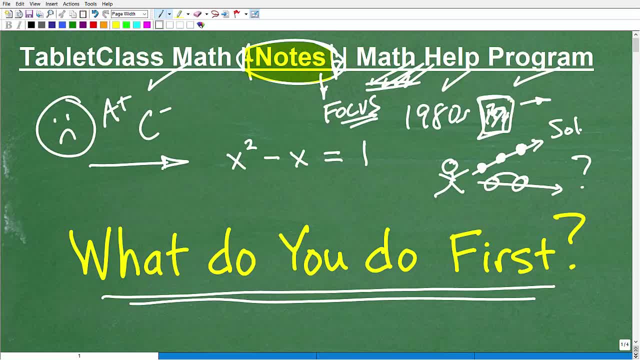 you do in life right, and math is no exception. now, in the meantime, you probably missed a lot of material uh that you still need to know, so i offer detailed, comprehensive math notes. you can use uh to include pre-algebra, algebra one, geometry, algebra two and trigonometry. you can find the 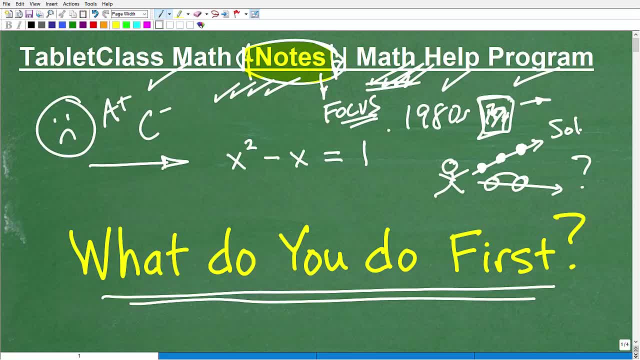 links to those notes in the description of this video. all right, so here is our lovely quadratic equation. that's what this is, uh, so, uh, what do we do? okay, now, if you think you can solve this problem, i would certainly encourage you to pause the video and go ahead and, uh, solve this, if you know what. 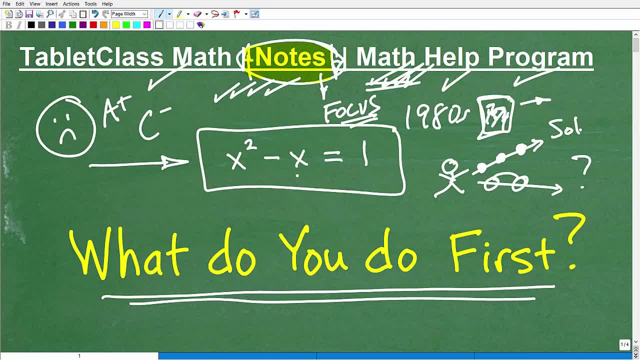 you're doing doing. you can solve this within- I don't know- 120 seconds. all right, two minutes. so this is not that difficult of a problem. but if you're not quite sure, I'm going to show you what to do right now. okay, so if you don't want to see the solution, go ahead and pause the video, but let's just very, very 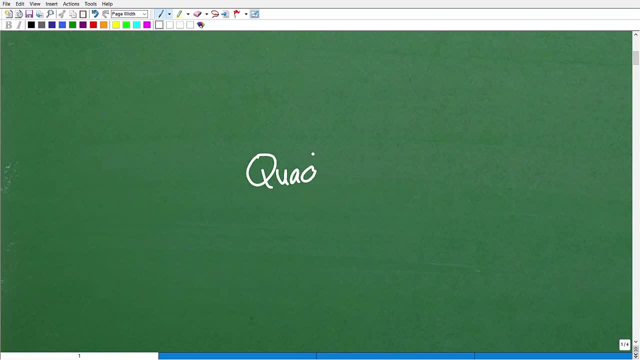 quickly talk about quadratic equations and some of our options. okay, so, depending on your, the way this quadratic equation is laid out- and I don't want to turn this into a full uh lesson on solving all quadratic equations because there's there's different types or there's different forms- okay, 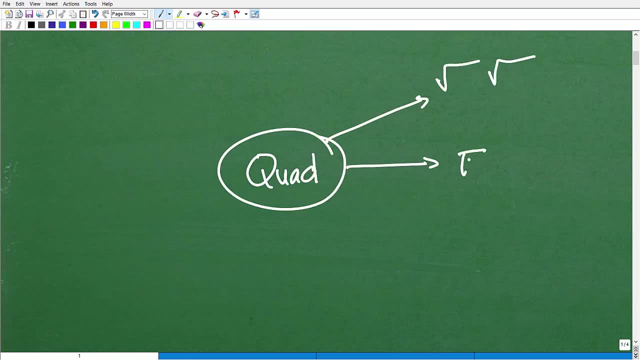 sometimes you can take the square root of both sides. sometimes you can factor. all right, now, when you can't factor or take the square root of both sides, then we have to go: uh, use some additional techniques, uh, to include the quadratic formula. okay, this is our fallback technique. and then 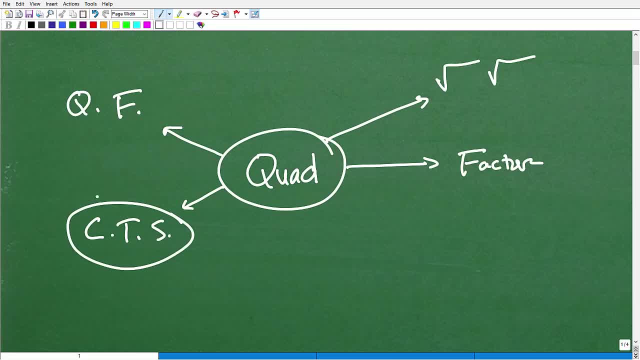 there's another technique that we're going to talk about in a little bit, but it's called completing, uh, the square, which is like the long version of the quadratic formula. so, in general, this is what you know. you're kind of, your options are, uh, when you're dealing with quadratic formulas. 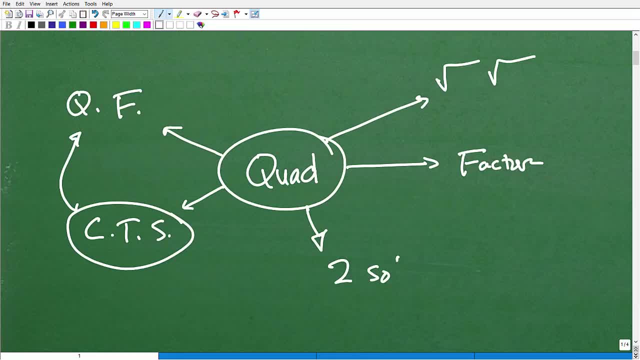 but one thing you need to know is that there are always two solutions, always two solutions when you're dealing with the quadratic formula. so any anytime you're dealing with an x squared. really, a quadratic formula, by definition, is a polynomial to degree two, so it is, in fact, a. 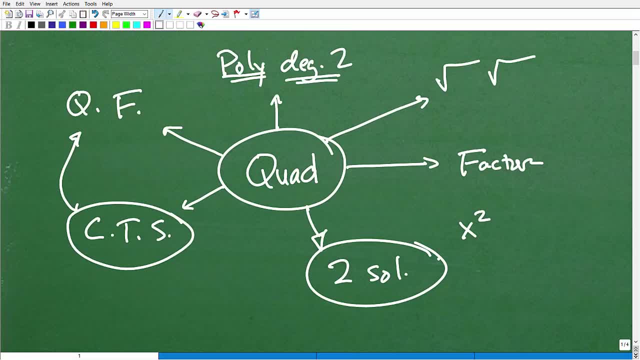 polynomial and its highest power is two. So you know, you've got to know this stuff right. You just can't be like: oh you know, I do this, I do that. You can't learn math by just memorization. 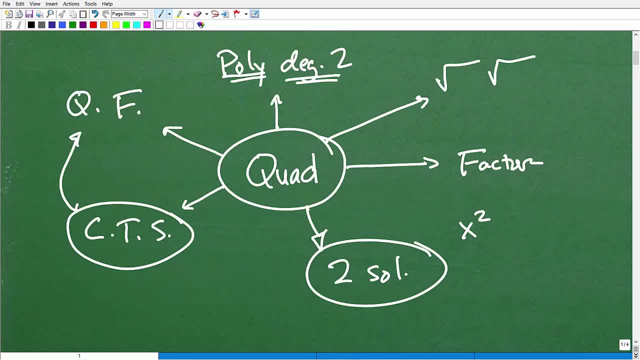 You've got to actually know the concepts a little bit. So this is a quick, quick overview of quadratic equations in general. Now let's get to our problem and talk about that first step, Like what's the first thing we need to do? 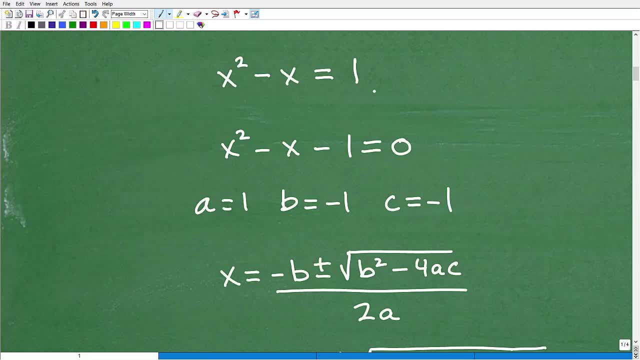 Well, this here's our problem, the first thing we need to do. okay, because this is not a situation where I can take the square root of both sides of the equation, all right, So here's a quadratic equation where I could just simply take the square root of both sides of the equation. 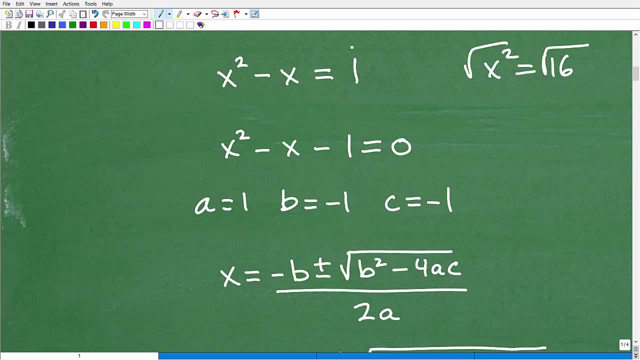 I can't do that because I have this x term, So I can't do that here. So this is not one of these scenarios. So I'm like: okay, I recognize I cannot do this, So what is the first thing I need to do? 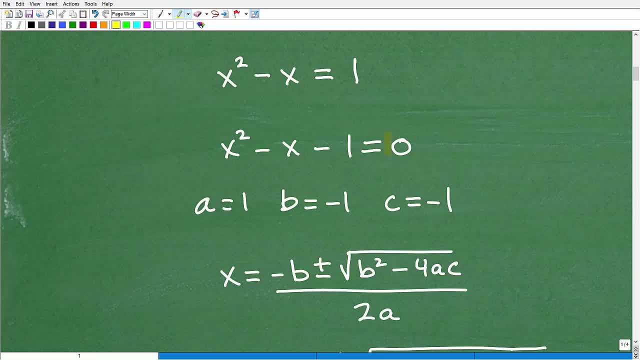 Well, the first thing you need to do is you've got to set this equation equal to zero, okay? So that's the first thing you always do in quadratic equations, Okay? Unless you can take the square root of both sides, then you're going to have to move whatever terms you have over on this side to the left-hand side. 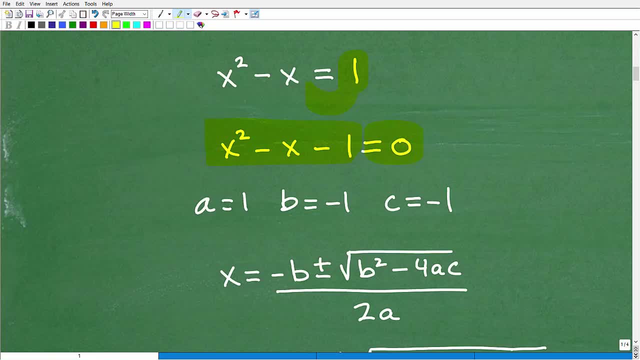 and have this in standard form. okay, You set it equal to zero. So really that's kind of like two things as part of the first step, right? So the first thing you want to do is set that thing equal to zero and then make sure it's in standard form. 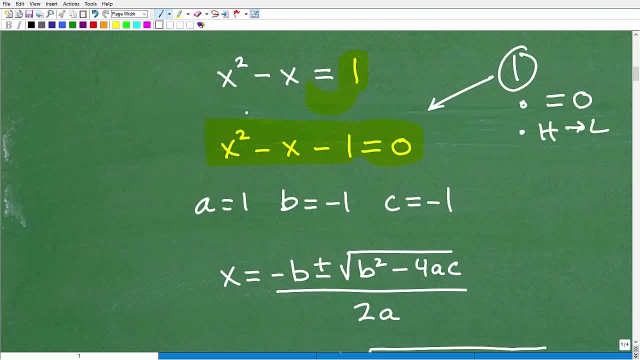 which it means that it's highest to lowest power. okay, So notice, here I have my x squared, my x and my number. That's the first first thing You want to do, unless, again, you can take the square root of both sides of an equation. 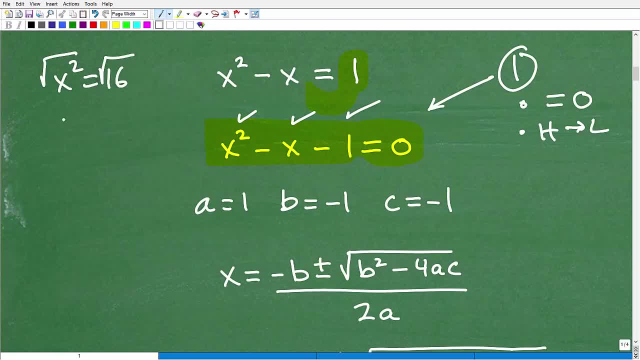 So like this: this is a quadratic equation. I simply take the square root: x is equal to positive and negative four, and I'm done All right. Unfortunately for you, this is not that easy. okay, All right. so that's the first thing. 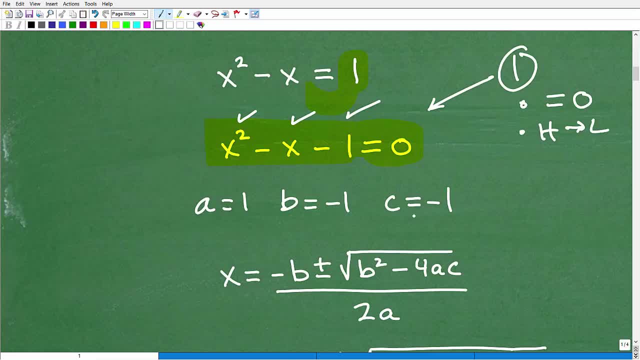 Now, what's the second thing? Well, the second thing. you can see I'm already doing a quadratic formula here, but the second thing would be to try to factor and once you're here, once you have this lovely trinomial, try to factor it, okay. 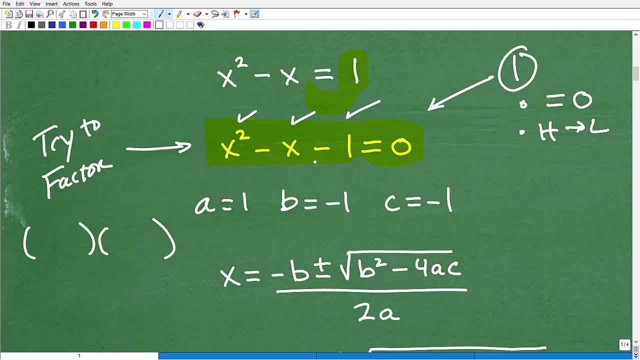 So, in other words, you're going to want to try to see if you can factor this thing into two binomials where it's that set equal to zero. Of course, you need to know a little bit about factoring, and that's a typical weak area for algebra students. 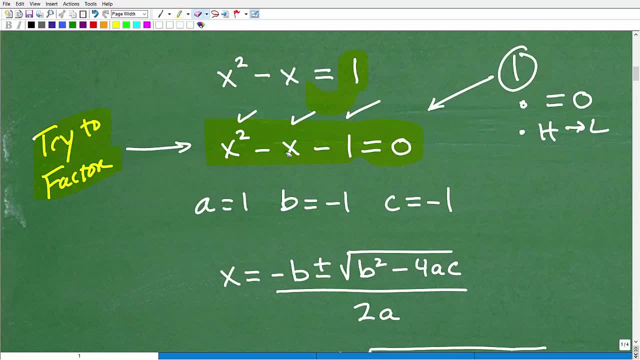 So that's what you want to try to do. okay, So you want to attempt to factor this? all right, So that's the second thing. Anytime you have a trinomial, your brain needs to be like: all right, can I do this? 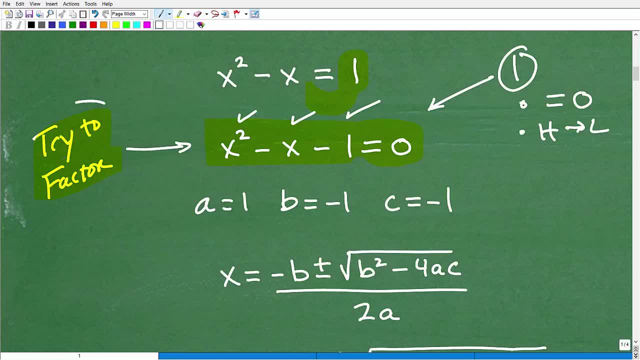 Can I factor this? and try to factor it Now, if you are struggling with factoring trinomials, I have tons of videos on my YouTube channel about factoring. You want to check those out or you might want to, just you know. 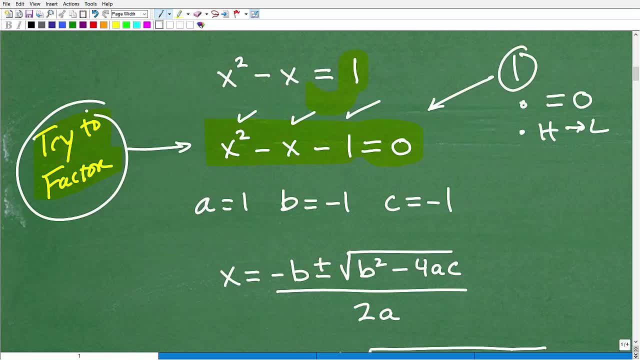 enroll in my Algebra 1 course and you'll just be like a total expert in this. But anyways, so that's the second thing. So the first thing: set this thing equal to zero. That's the first thing, right? Then the second thing is to try to factor this. 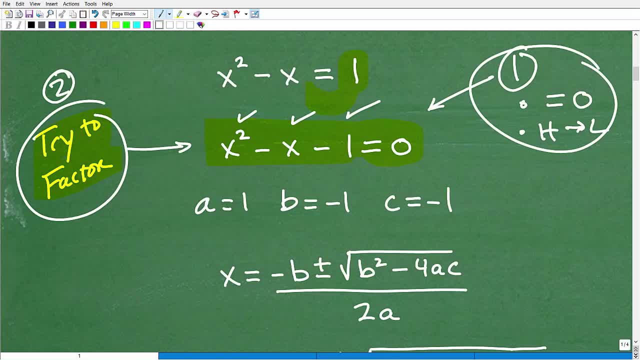 Now, unfortunately for us, this guy right here cannot be factored. We can't factor this into two binomials. So you know we're like: oh bummer. You know what do I have to do? Well, you're going to have to break out the good old quadratic formula. 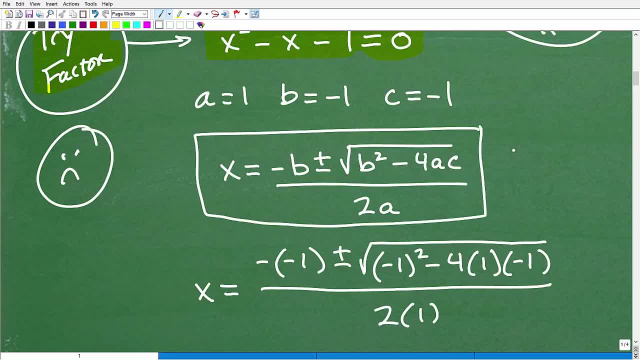 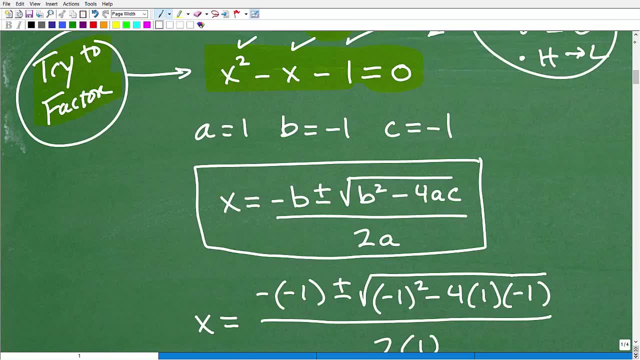 Here it is right, here, in all its glory. This is one of these things you want to put into your long-term memory. okay, It's that important, So you should know this. but if you don't know this, here is the formula. but we need to know how to use it. 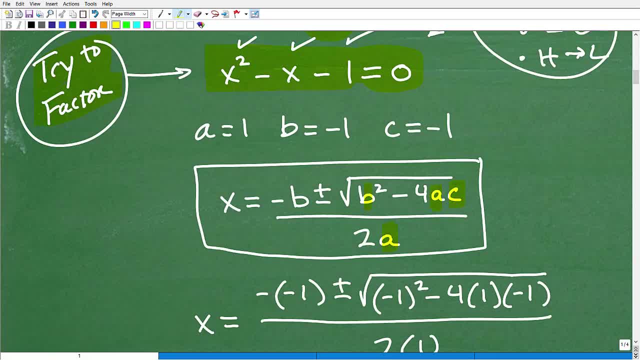 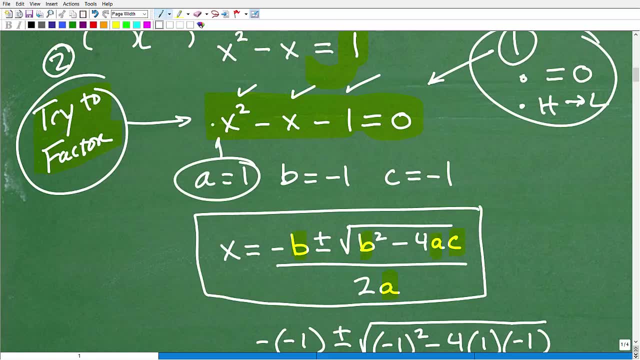 So what's in the formula? We got A, We got a C, We got some Bs here. So what are ABCs? Well, A is the coefficient of that leading term. okay, We call it the leading coefficient. So whatever is in front of the X squared, in this case it's a positive one. 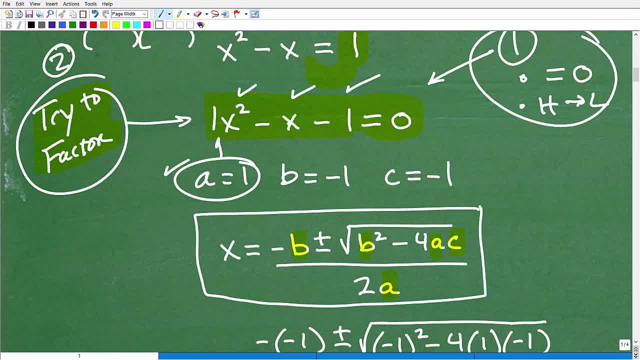 That's what A is equal to. Whatever is in front of the X term, in this case it's negative one. That's what B is equal to, And then our little number by itself, that's what C is equal to. So C is negative one. 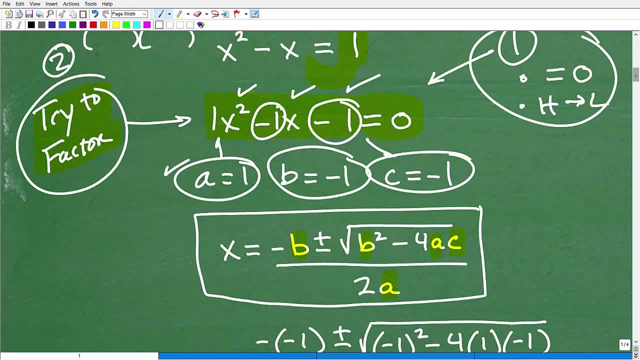 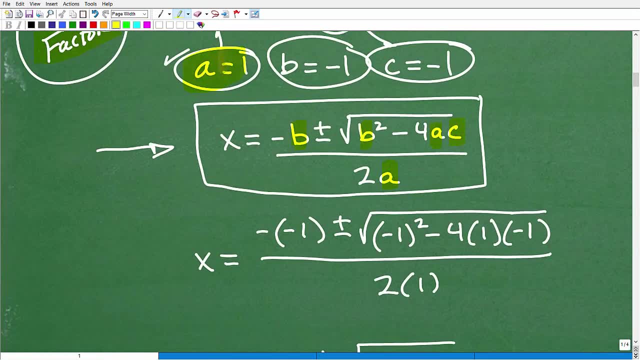 B is negative one And A is one, okay, So now we plug in those respective ABC values into the quadratic formula And you can see here: A is one, So that's going to be right there for my one, And then B is negative one. 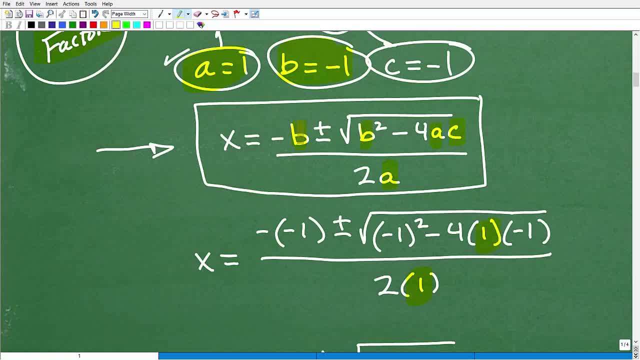 You've got to be very, very careful here. B is negative one, So the formula is minus B. So this is minus a, minus one, okay, Or negative of a negative one. B squared here, that's negative one. squared Minus four times A times C is negative one, right there. 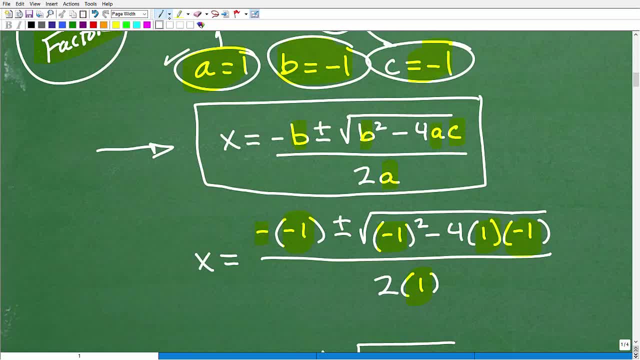 So you've got to be very, very careful here as well. Now, when you work in a quadratic formula, once you- you know- have plugged in your values, do not continue At this point. you've got to stop yourself, okay. 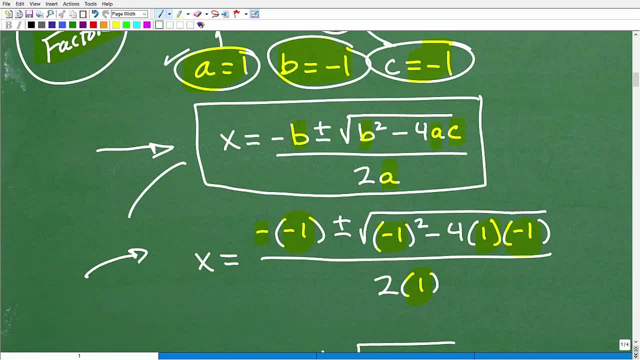 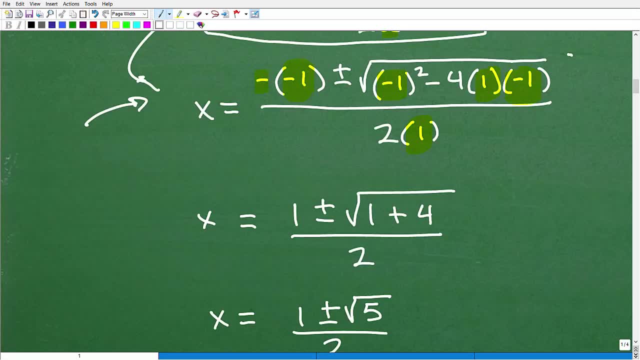 Because so many students make mistakes plugging in the values. So double, triple check that you've got all these values right And from this point forward you're going to have to be super careful that you don't make any little arithmetic mistakes. 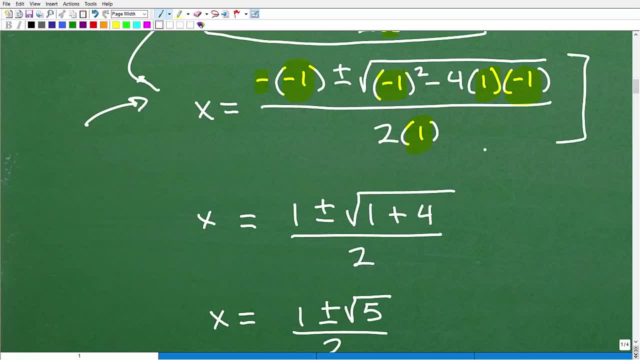 Because you know how many quadratic equations have. you know a number. Have I problems? Have I graded between homework, tests and quizzes? I believe about 100 million. okay, Now, obviously you know, over decades of teaching mathematics have I really seen 100 million quadratic equation problems? 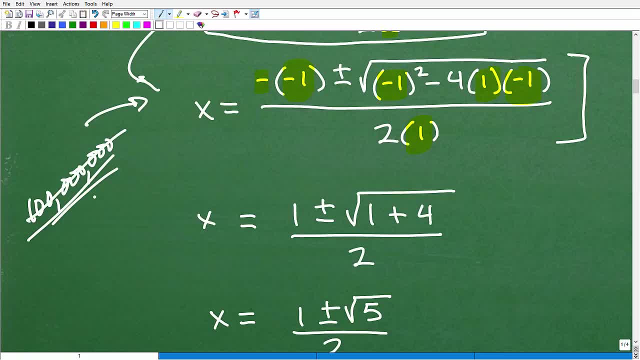 No, but it's a lot okay. So you know, I'm like a machine. My eyes are like: okay, I know exactly what to do. I'm like a little like advanced computer program, Like okay, da, da, da, da, da, da da. 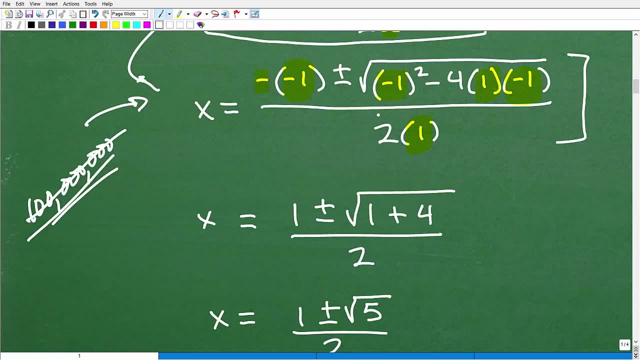 I'm like a, I'm like a machine, I'm like a robot. I'm like a robot. I'm not like a robot, I'm like a. you know, like a robot. And then you know, I found out about the bionic man. I found out about that guy back in the 1970s. What was that? robot guy, Bionic man, That's the name of him. If you're not familiar with that, check out that guy, the bionic man. all right. 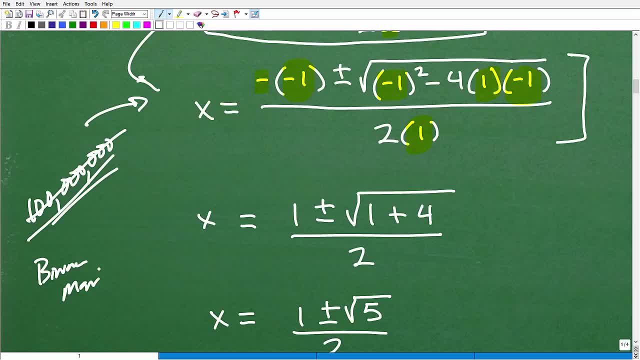 So he was very cool. He had all kinds of like bionic features. That's how I was, because I was grading so much work. Any teacher would relate to that. But anyways, you know my senses are on high alert. I know exactly where students are going to make errors. 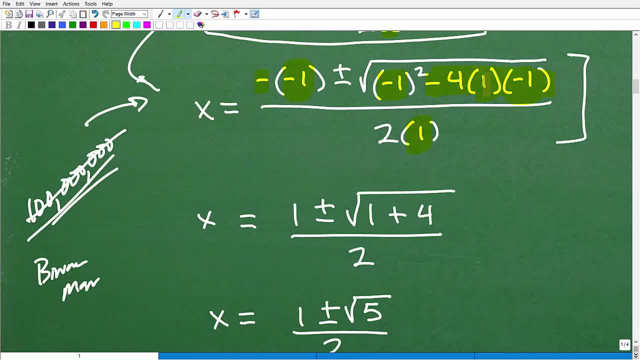 So you've got to be super careful in here. All right, This is the negative. four times one is going to be positive. basically right, that's going to be a positive four negative one squared is one and then minus, minus one is one and we have a plus or minus, and then two times one is two. 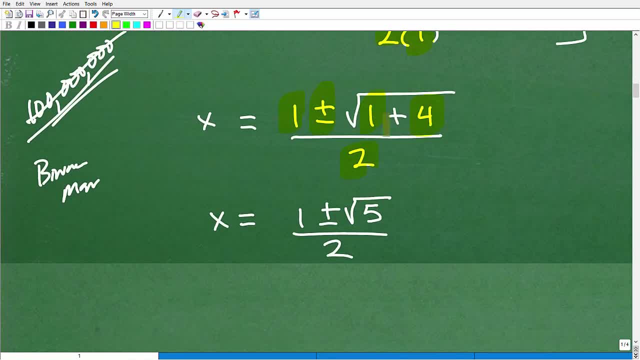 and i'm kind of going quickly here again, you need to practice the quadratic formula. i have tons of videos on this in my uh algebra playlist on my channel. so one plus four, that's five. so one plus or minus uh two. this is the final answer. now i said there's two solutions, so hey, uh, mr youtube. 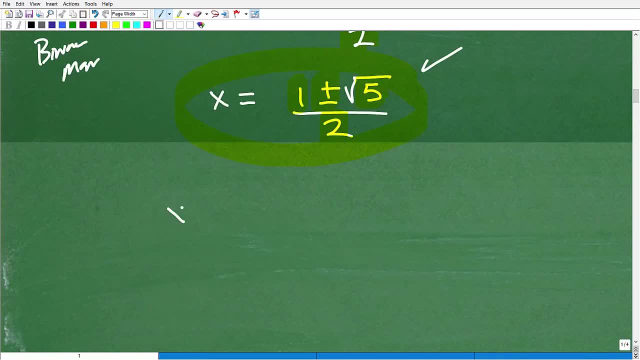 man, you said there's two solutions. this is just one answer. well, no, the first answer, this little plus or minus, means one answer. you're going to go one plus the square root of five over two. that's one separate number. okay, the other number is one minus the square root of five. 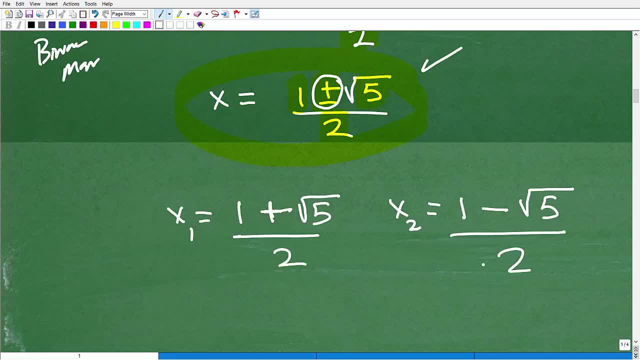 over two. okay, so instead of writing these two answers this way- what we do in mathematics is very, very common- we just combine these guys, we squish them together and we're like: look, this is a plus, this is a minus. we'll call it a plus, or? 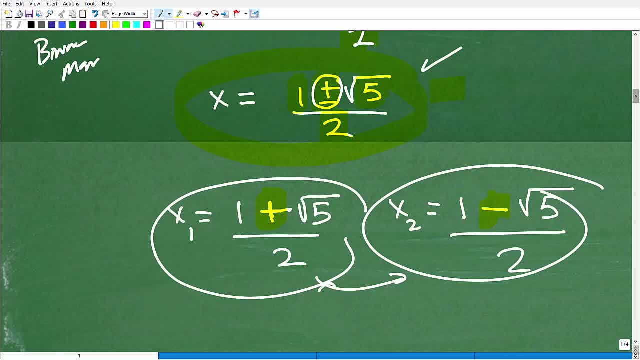 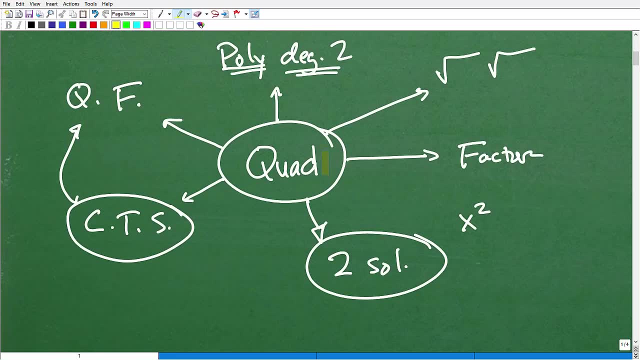 minus and just write the same numbers. okay, so that is that again. quadratic formulas: tons of stuff you need to know, right about quadratic formulas. right what they are? they're a polynomial degree two. they're always going to have two solutions. sometimes we could take the square root of both. 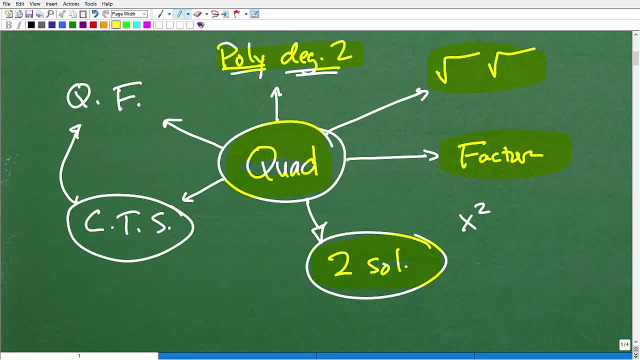 sides. sometimes we can factor, okay, but when none of these options work, we have to fall back on the quadratic formula. and again there's this thing called completing the square, which is like the long version, but you're going to need to know how to do this as well. all right, so just just a quick. 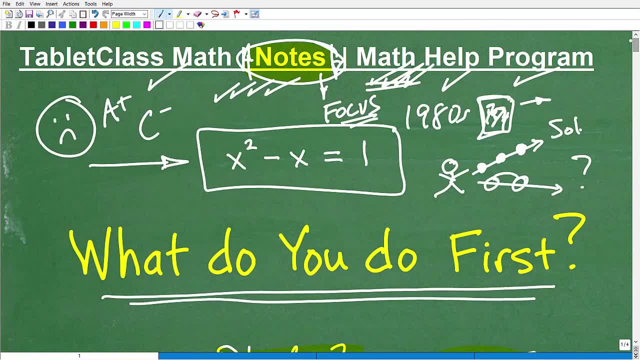 overview of quadratic formulas. now, if, in fact, you got this problem right and you understood everything i was talking about, then i must in turn give you a happy face with a mohawk and a plus 100 and i'll give you a couple stars there, um, back in the good old 1980s, uh people, in fact. 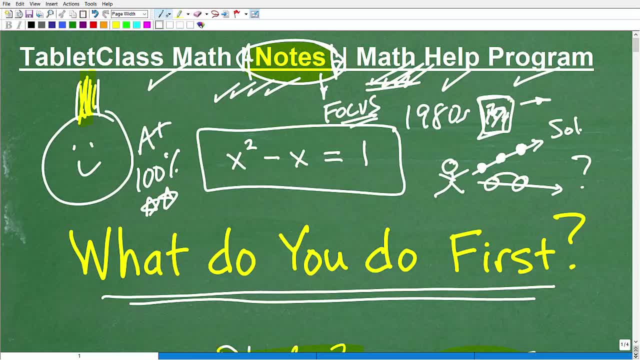 did have a happy face and they did have a mohawk and they did have a mohawk and they did have a have Mohawks. we used quite a bit of hairspray. It was probably pretty dangerous to use that much hairspray in your hair back in those good old days, But anyways, we thought we were cool. I